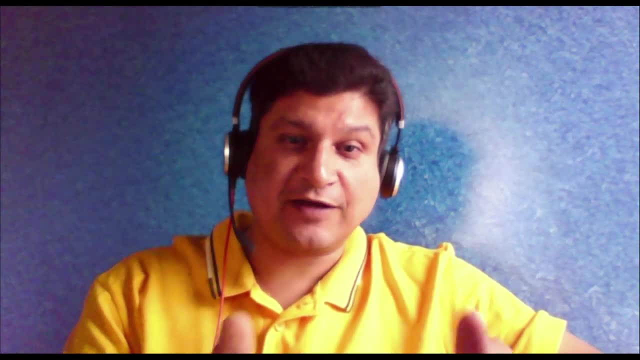 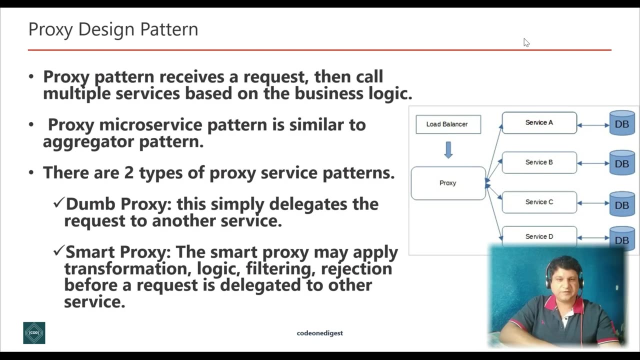 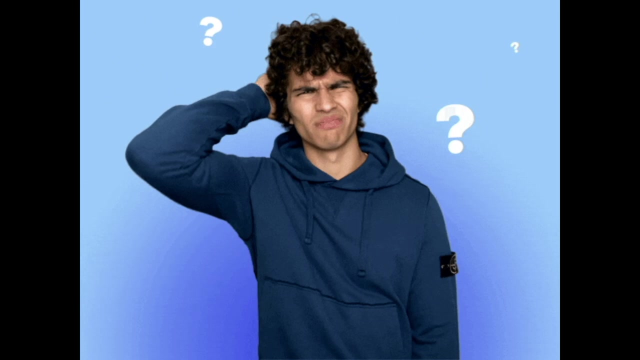 subscribers. i want you to like, share and subscribe my channel so that i can grow code one digest family. thank you, oh, i'm so excited. okay, friends. so now let's start with the proxy design pattern. so let's understand what is proxy design pattern? remember, this is the third design pattern, integration design pattern category for. 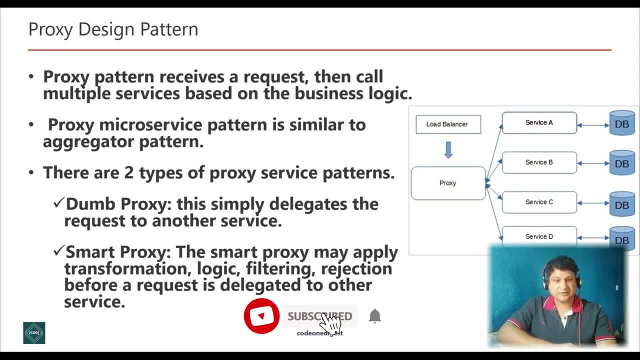 microservices. proxy design pattern is a variation of aggregator model. in this model, we will use proxy module instead of aggregation module. proxy services may call the aggregator model. in this model, we will use proxy module instead of aggregation module available. in this module, we use proxy module. i think we raise it up so that we can provide. 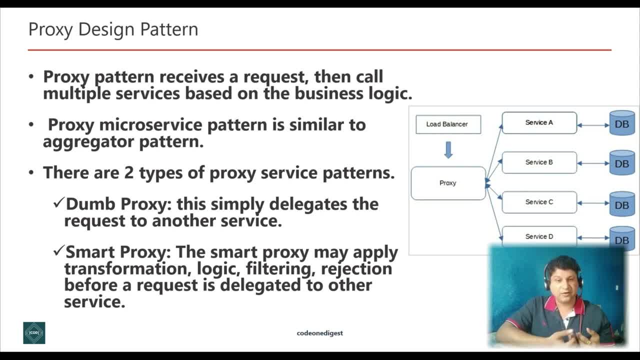 different services individually in proxy pattern. we can build one level of extra security by providing a dump proxy layer. the proxy service pattern can be subdivided into two categories. one is dumb proxy. this is simple: the delegation of request to another service. then next is smart proxy. the smart proxy may apply some transformation, some business logic and 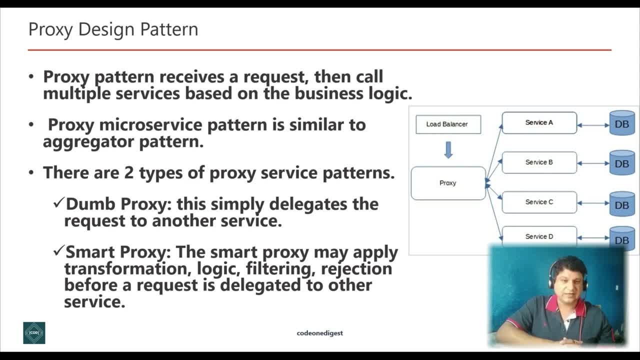 filtering and revision of the proxy in a one layer for two categories. the next is smart proxy. we might apply a transformation, some business logic and filtering and rejection before the request is delegated to other service. So in this smart proxy we may do certain transformation. 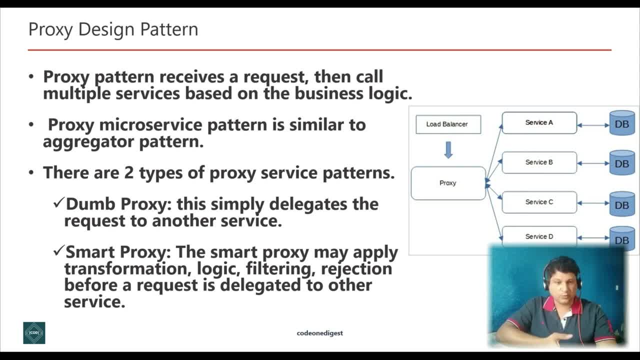 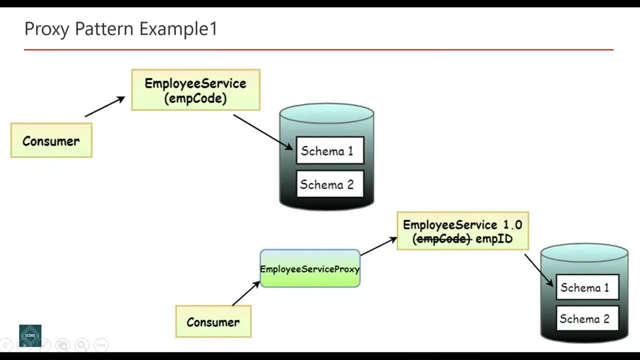 There may be some logic to filter and reject the request before we delegate it to other service. Let's understand this design pattern with a real world example. We have an employee leave application example that you can see on your screen and we'll understand the proxy design pattern. 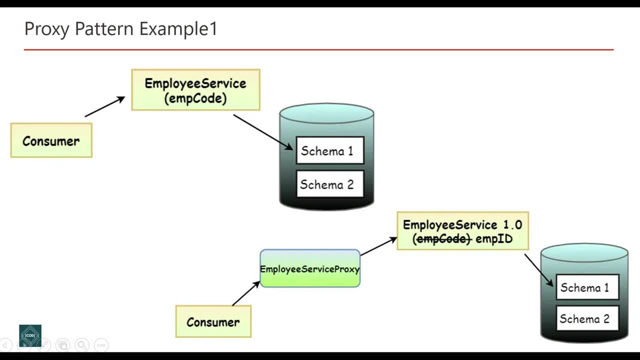 with this example. Consider: you have a microservice to get a leave information of employees, So the consumer need to pass the employee code to get leave information. But soon, with the new restructure in your organization, you have decided to keep employee ID as a relational key. 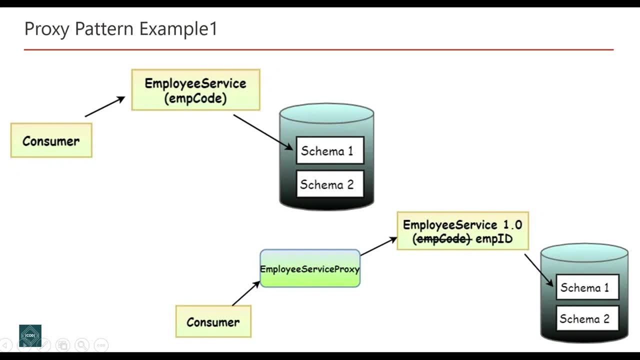 for all the records instead of employment code. So if we deploy new restructure employee service, new version of the employee service, so it will not work for existing consumer who are calling the service by passing the employee code Right, Because those consumer will pass the employee code. 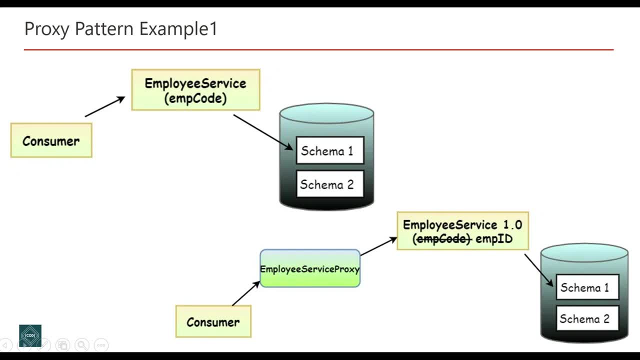 as the input to get data, But the newer version of service expects the employee ID as the input. So as a solution for this, we can use the proxy design pattern in this scenario. Proxy microservices services design pattern is slightly similar to the aggregator. 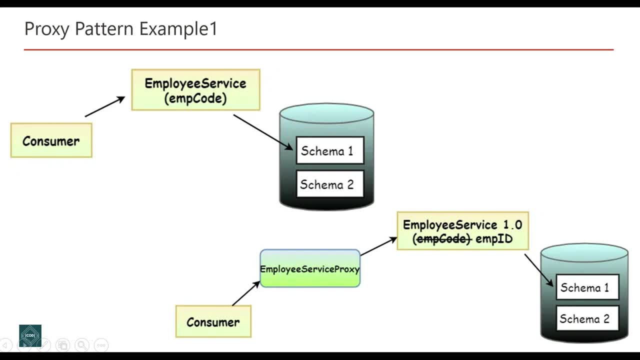 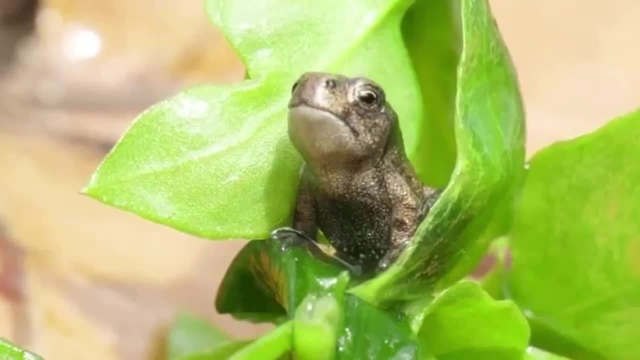 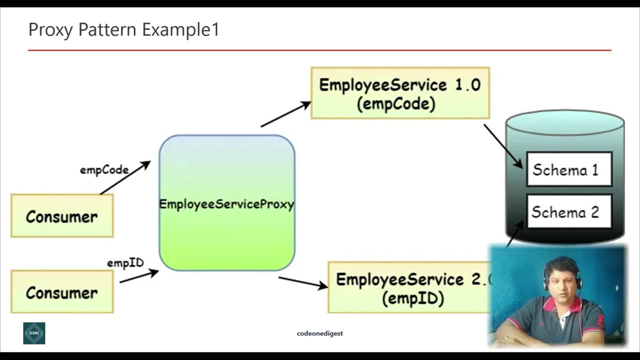 but instead of aggregating the response from various services, this pattern makes call to other services based on the business requirement Really. So we can solve the problem by creating a separate proxy service. So in a new solution, the consumer will invoke the proxy service. 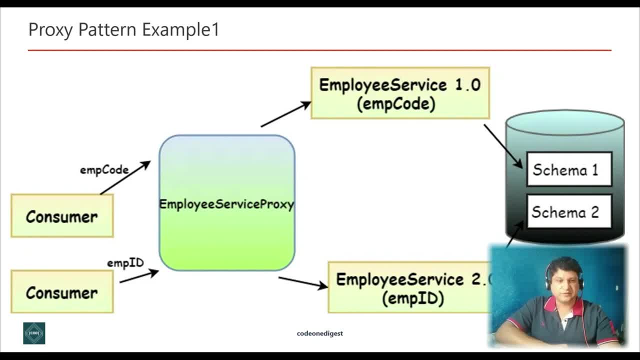 if the consumer passes employee ID, So proxy service will call new version of the service. But if consumer passes the employee code, then proxy service will call the older version, one based on employee code. So in this way you can independently deploy the services. 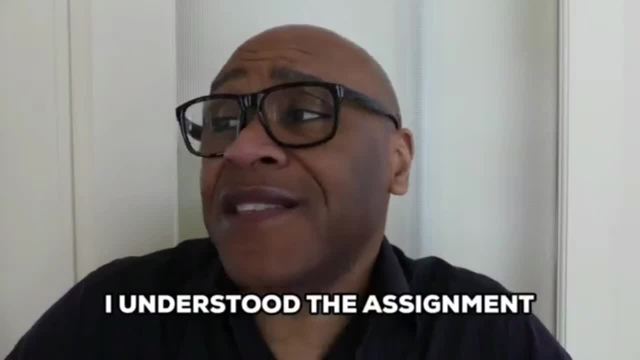 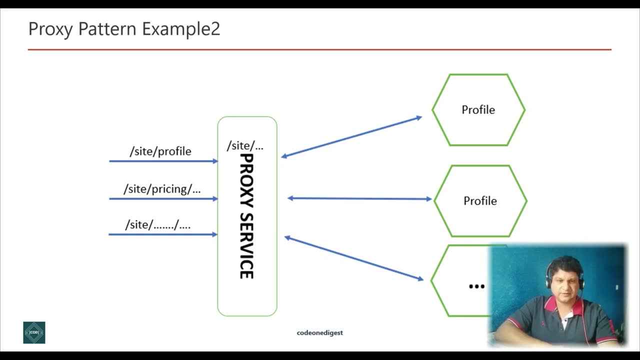 without affecting the consumers. I understood the assignment. Let's take another example of e-commerce application to understand the proxy design pattern In this example: e-commerce application, where you are only interacting with the UI and access all the resources via API gateway. 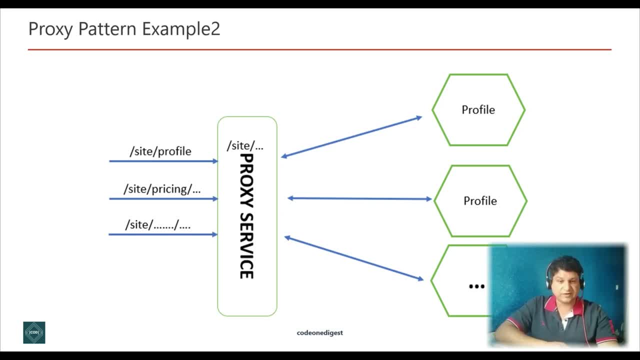 that is proxy In the background. the different functionalities are served by different services like cart and voicing and so on. Also. another good example of this would be the various presentation layer for different devices. Presentation layer only call proxy service and proxy service called devices specific services. 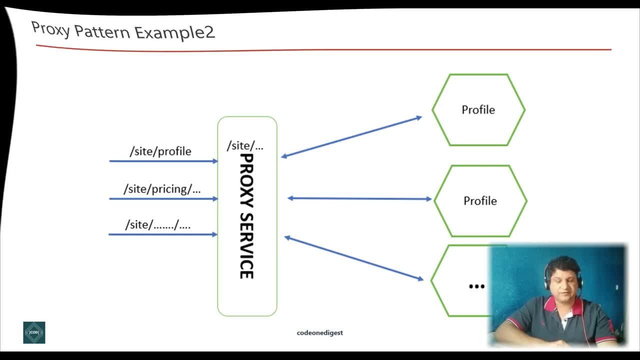 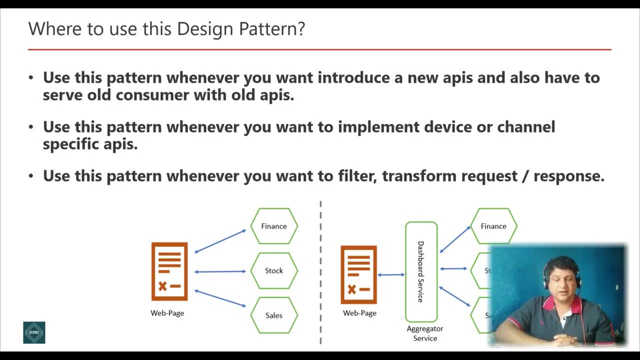 like mobile app, website or TV. Yes, that's amazing. So what are the use cases of proxy design pattern? How can we use it in our project? In which conditions we can use proxy design pattern. So let's understand that. 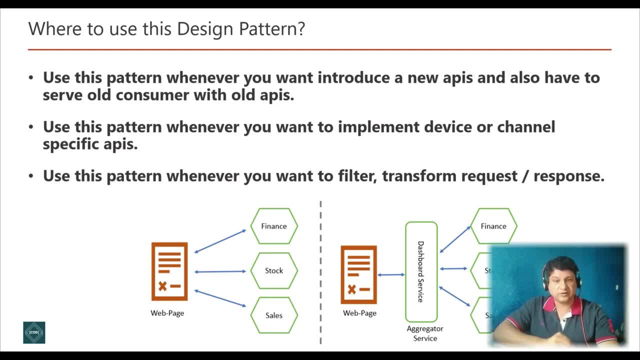 Whenever you want to introduce a new API and also have to serve your existing consumer base with old API, then you can choose to use proxy design pattern. Whenever you want to implement device or channel specific APIs, that time you can use proxy design pattern. 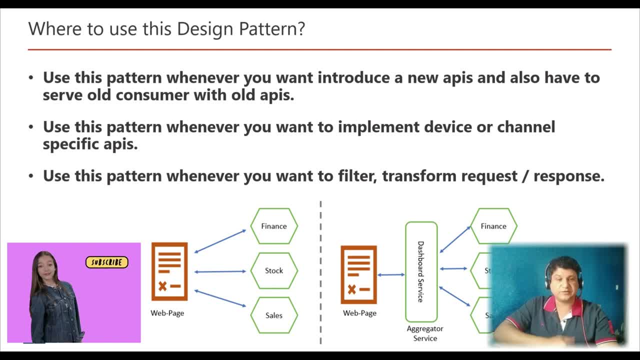 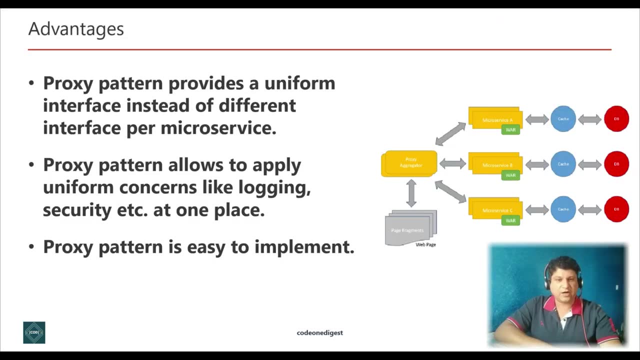 Whenever you want to filter or transform requests and response based on certain logic, that time you can use proxy design pattern, where you can have that logic to filter or reject requests. Right, Friends? what are the advantages we get out of proxy design pattern? 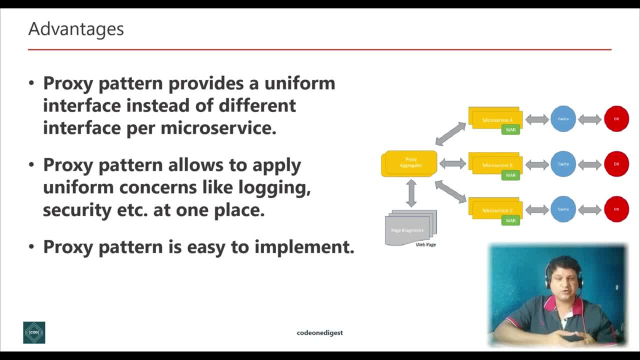 Let's understand that before we actually use it, we should know the value that we are bringing in on a table using proxy design pattern. So proxy design pattern provides a uniform interface instead of different interface for microservices. Proxy design pattern offers you a single API. 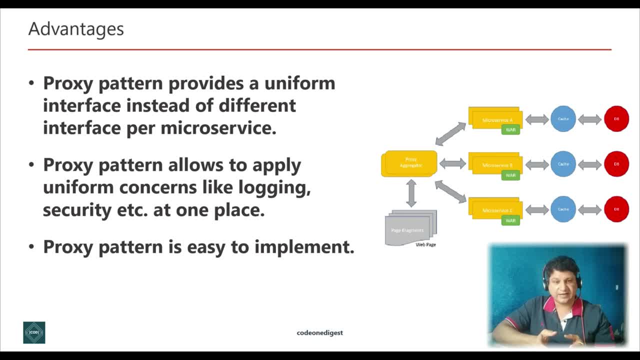 for all your consumers and let the proxy decide where to route this incoming request. based on business logic, Proxy pattern allows to apply uniform concern like logging, security, et cetera, et cetera- one place. proxy design pattern is very simple and easy to use. using proxy design pattern, we can. 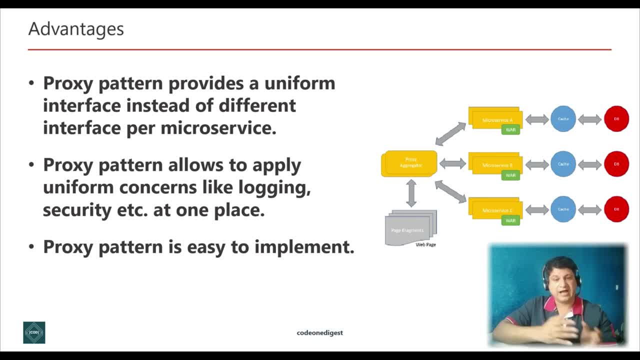 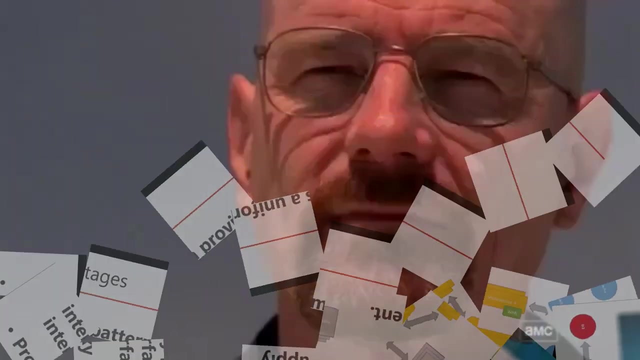 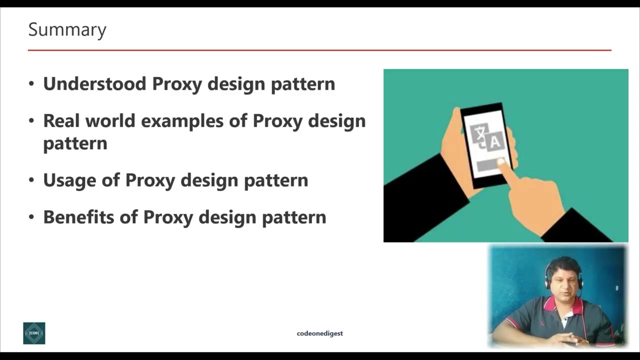 maintain the multiple versions of api and support our old consumers which are using our old apis. we can use proxy design pattern for validation and security purpose. the validation and security associated with the external service can be implemented and can be encapsulated easily in a proxy right. you're goddamn right, friends. now let me summarize what we learn in this video. 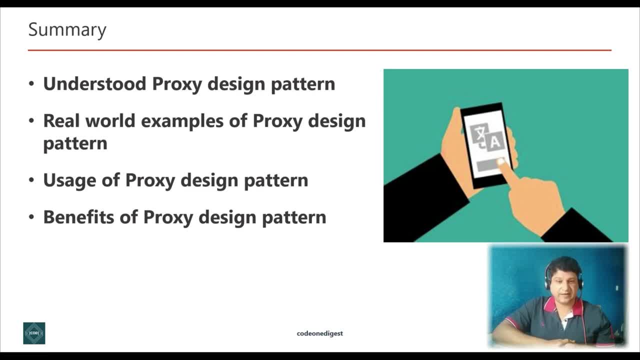 i gave the introduction of proxy design pattern. what is proxy design pattern? then we saw real world examples of proxy design pattern. what is the use of proxy design pattern in which scenario we can use the proxy design pattern? then i explain you the usage of proxy design pattern. 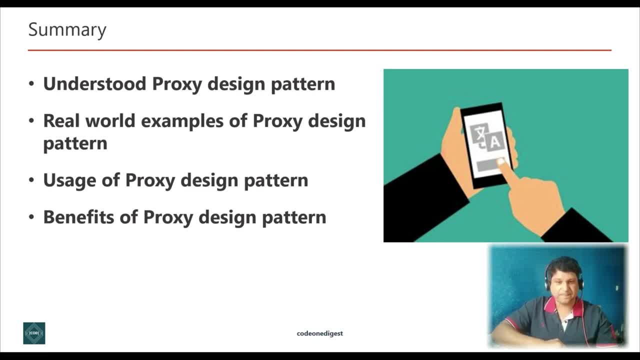 in the situation where you're using a proxy design pattern is the right fit, then i gave you the benefits and advantages of using proxy design pattern in our project right. so, friends, let me know if you have already used this design pattern in any of your project or seen a scenario where this pattern can be very useful. please provide your answer in the